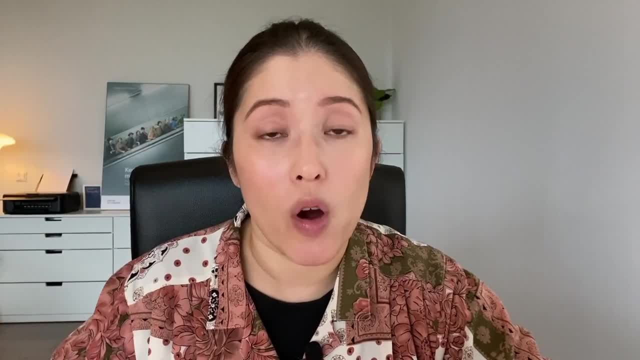 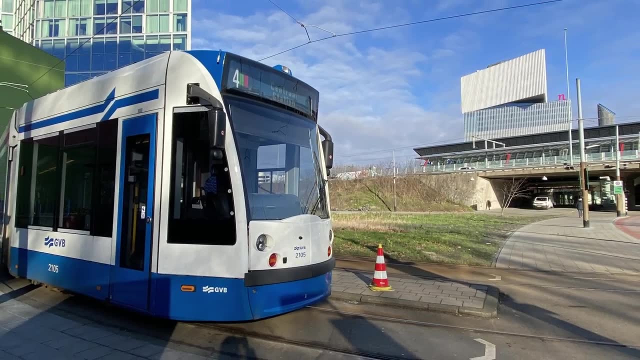 but you can normally gain entry at the door next to the driver, and then there'll be a door sort of near the end of the tram for getting in as well. When you need to get off, ring the bell in good time. identify a door that you can exit from. 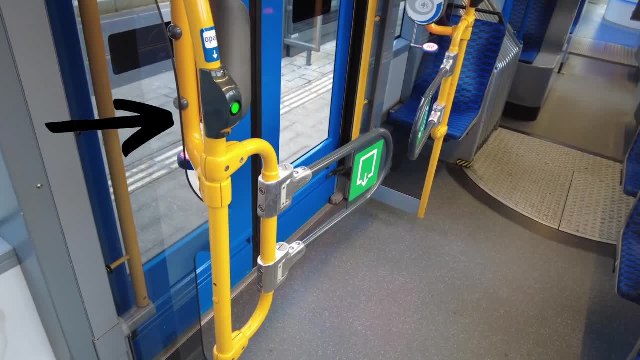 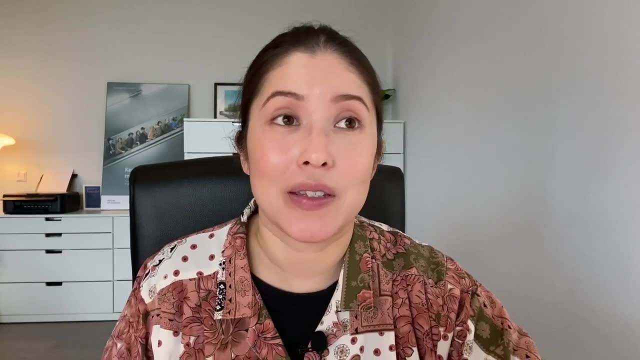 and make sure you press the button on the handle near the door. Now, if you don't press that button, the doors won't always open, And I've seen so many people do this. I've done this myself, You know. the doors don't open. and then there's this mad dash to the next set of doors. 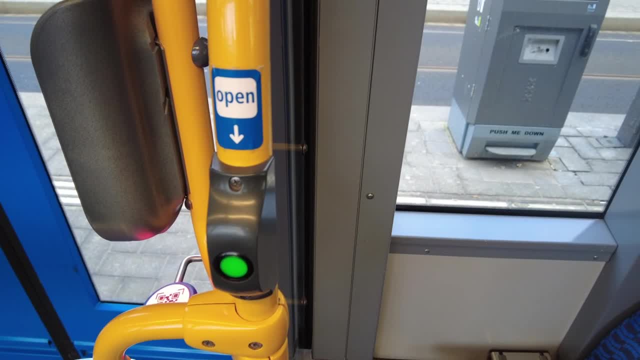 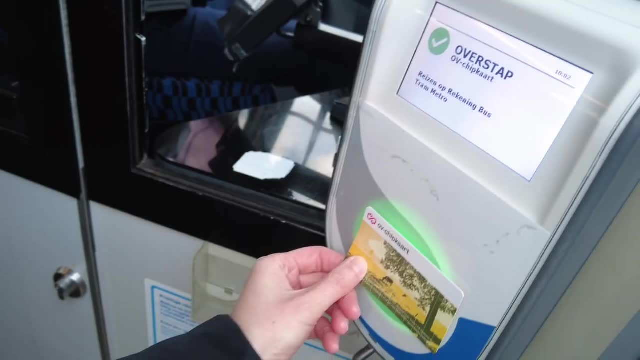 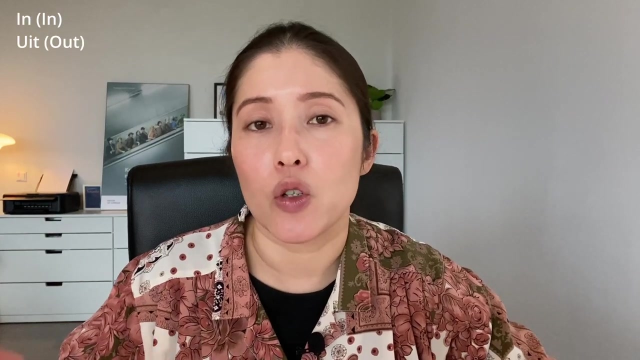 So embarrassing. I've noticed more and more that there are these open stickers next to the buttons now, but not all the trams have them. Definitely something to watch out for. When you board the tram, you need to tap in with your ticket And when you leave, you need to tap out And you'll see the words in and out. 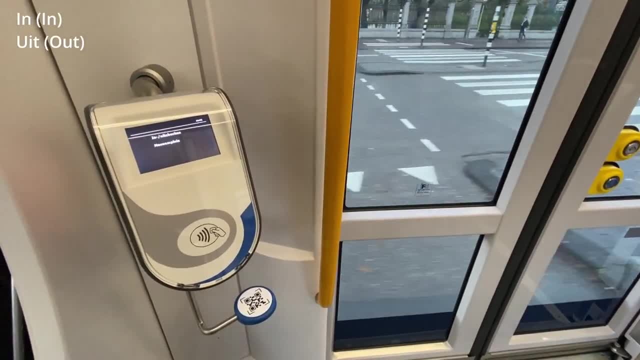 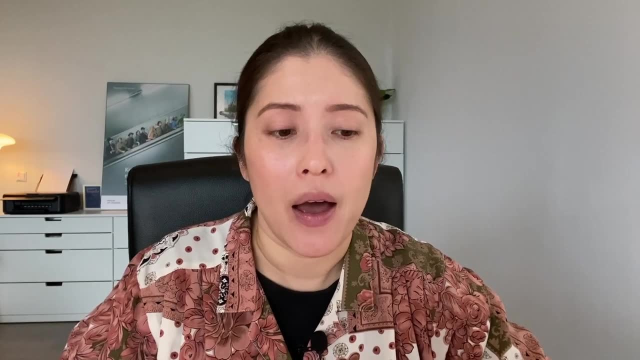 on the ticket reader. These machines can be a little bit temperamental sometimes. So yeah, if one machine doesn't work, just try another. Sometimes you might also accidentally double tap, So always make sure as you leave it says out Bus In terms of boarding the bus. 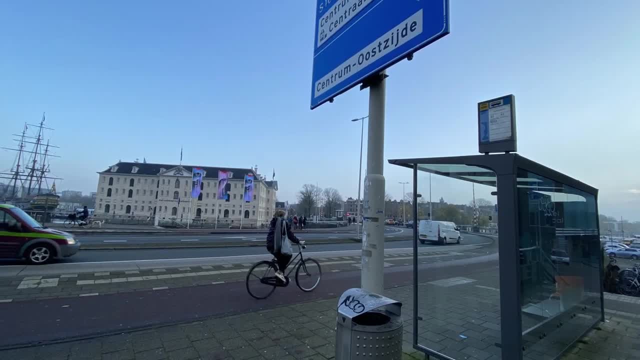 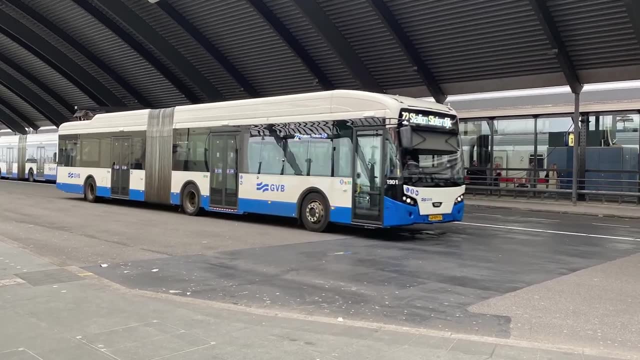 you normally board near the driver, but sometimes you can board the other doors too, Just like the tram. you need to tap in and tap out with your ticket When you need to get off, ring the bell in good time and get off the bus using one of the rear. 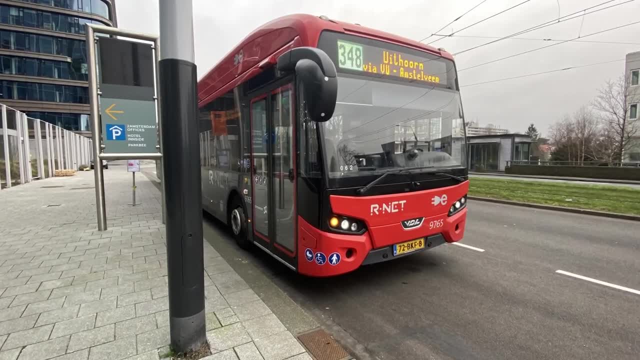 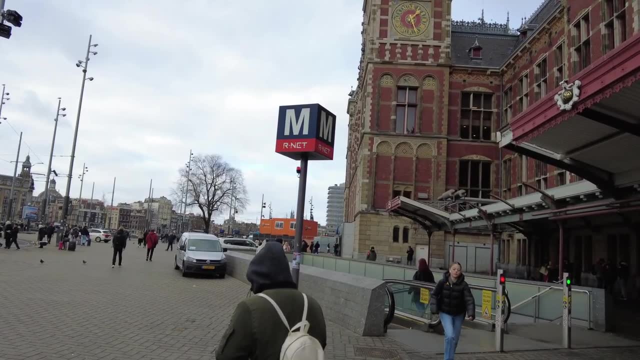 doors. You may also see some buses that are of a different color, and these are run by different companies and serve suburban and regional areas. Metro, The metro, is very straightforward If you are new here and you've got a choice between the tram, bus or metro. 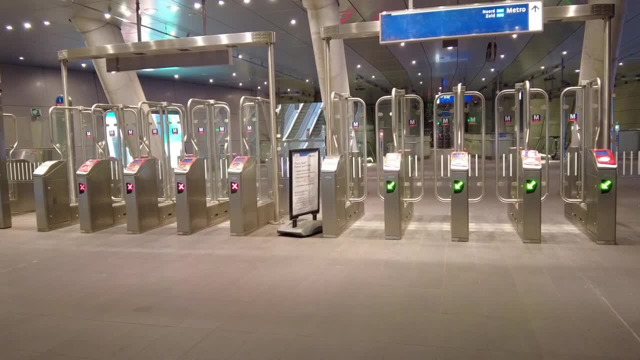 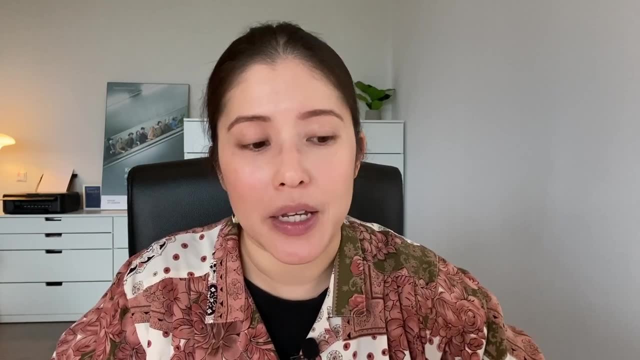 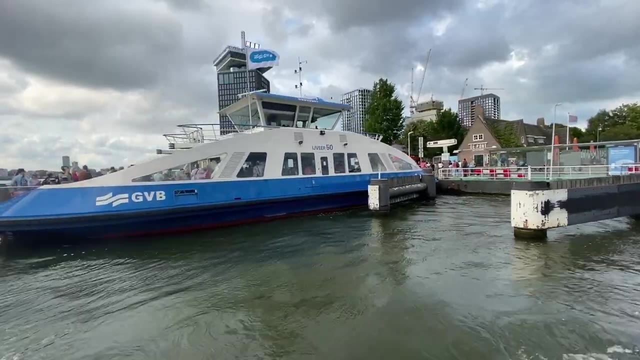 I would stick with the metro. Ticket barriers are very clear And again, you need to tap in and tap out. The metro will stop at every station And the only thing that you need to worry about is pressing the button to open the door. Ferry: The ferries F1 to F7 are completely free to use. 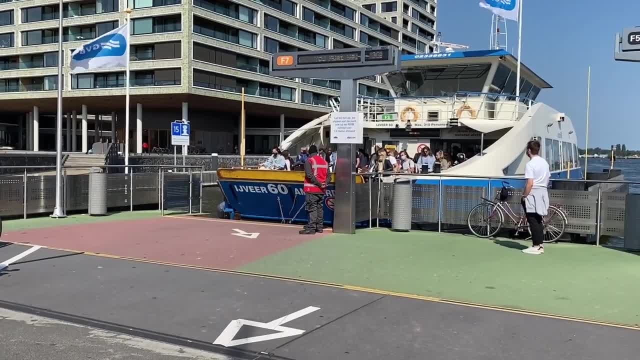 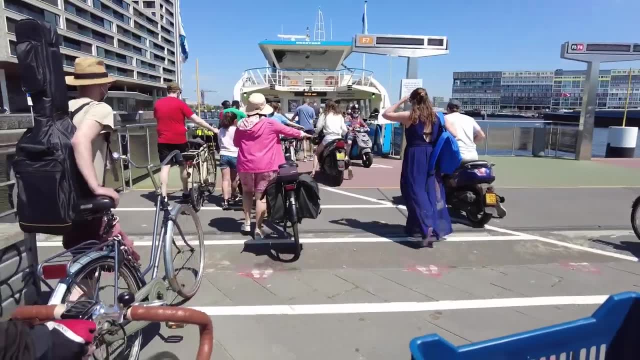 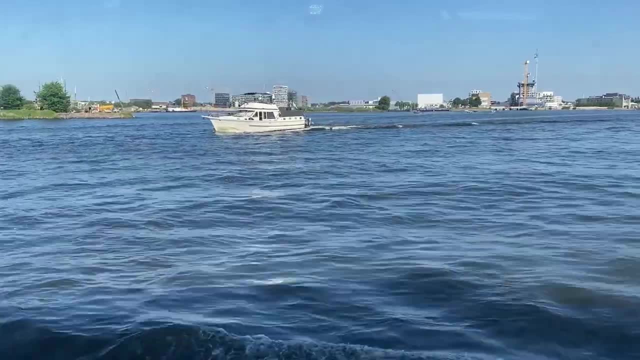 There are several ferry routes, but essentially these ferries are connecting the center bit of Amsterdam with Amsterdam Nord, because in between you have the River Ey. So you'll see pedestrians, cyclists, mopeds and sometimes even small cars on these ferries. Journey times vary. 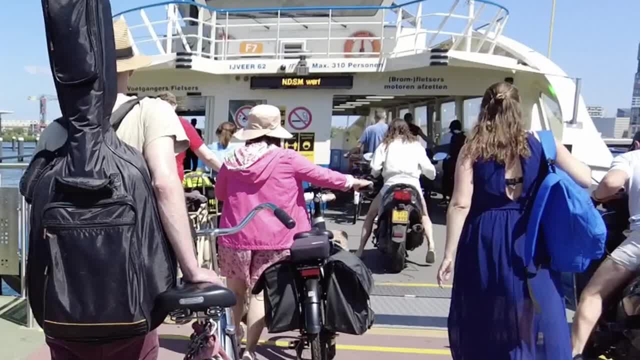 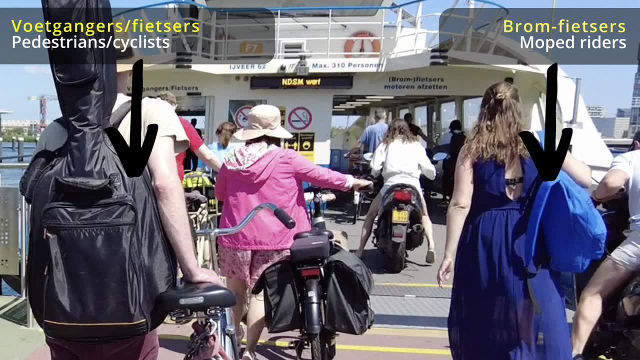 a few minutes to a maximum of about 15 minutes. When you board the ferry, there are two separate areas. One is mainly for pedestrians and cyclists and the other is for motorized vehicles. Just before we go any further, if you are getting any value out of this video, 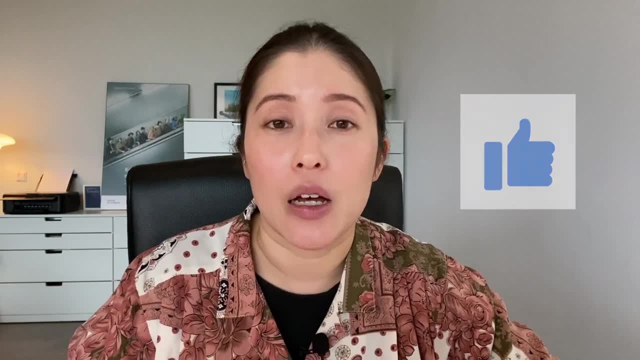 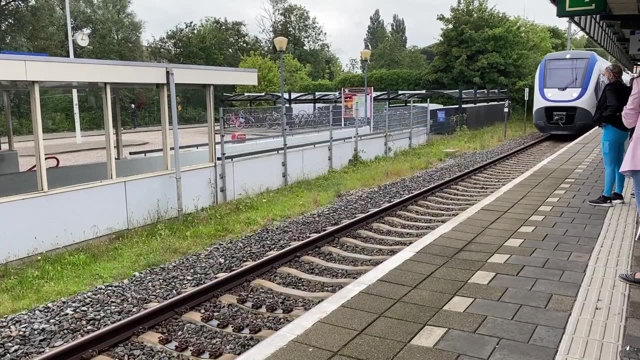 please do me a favor and hit that like button, as it really helps. small channels like mine get noticed by the algorithm. Thank you so much. Train. The Netherlands has a very extensive railway network and it's very easy to get on and off the train. It's very easy to get on and off the train. It's. 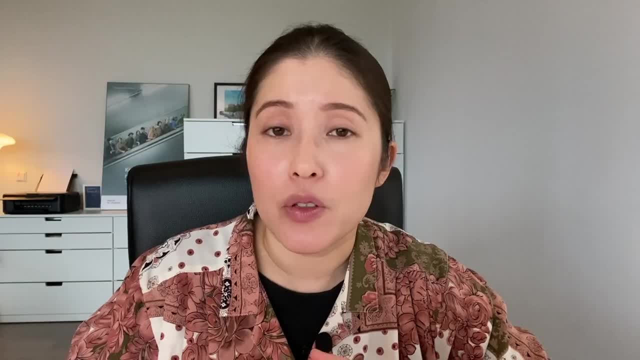 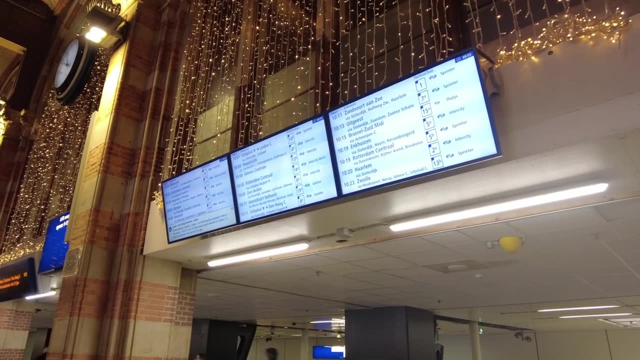 run by a company called NS. There are different types of train. For example, you have a sprinter train, which will stop at every single stop. There's also an intercity train that will only stop at major stations. Some trains are single decker, others are double decker. 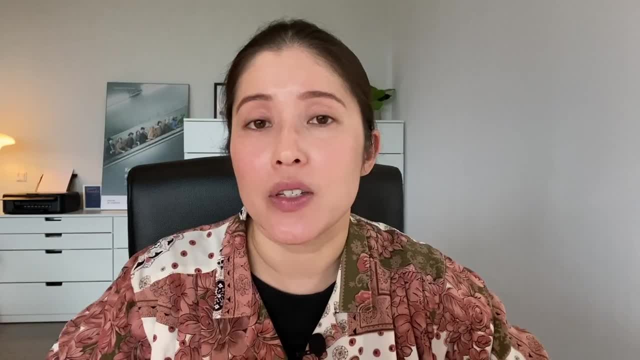 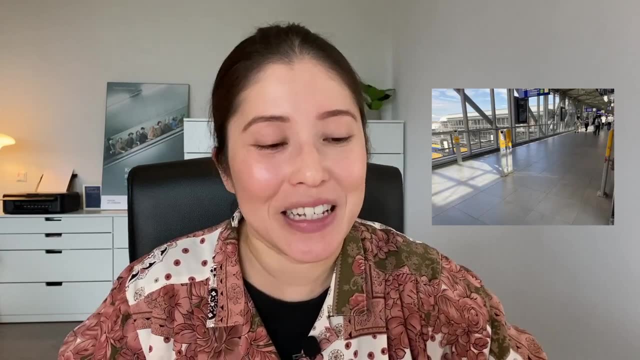 You will need to tap in and tap out with your ticket. In terms of ticket barriers, you have the standard looking ticket barriers, but you also have this type of barrier where you- I guess you- actively need to remember to tap in and tap out yourself. 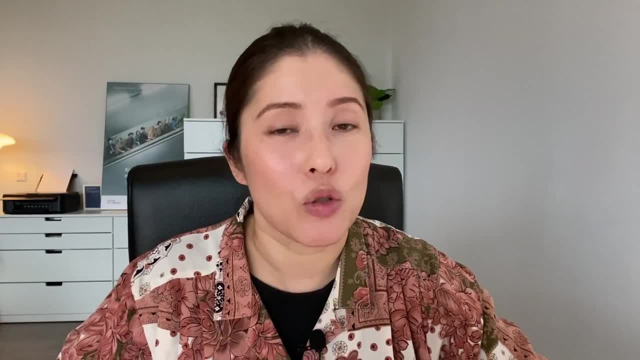 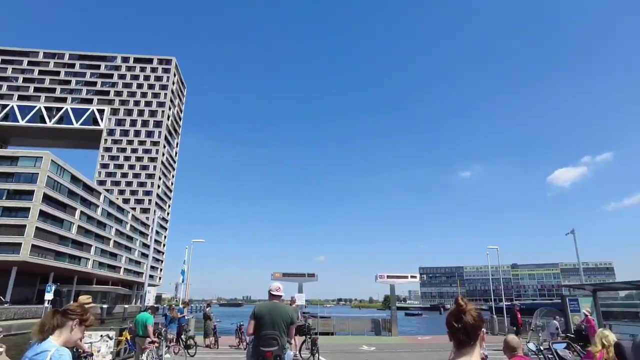 Tickets. Now there are so many different types of tickets that you can buy. Honestly, it's a little bit confusing. If you are staying in central Amsterdam, here are some ticket options for you. First of all, you have the GVB ticket, which gives you 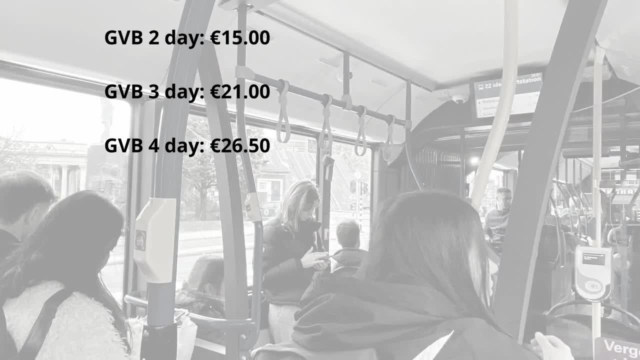 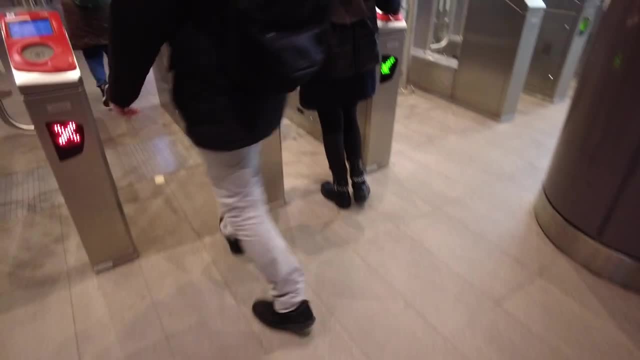 unlimited travel on the bus, tram and metro. It varies in length of time from one hour to 24 hours, right up to seven days, and it's activated the first time you tap in. For the 24-hour ticket: you can buy this in a 24-hour ticket. For the 24-hour ticket: you can buy this in a. 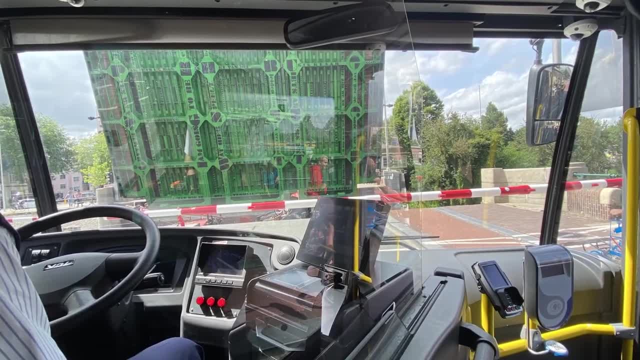 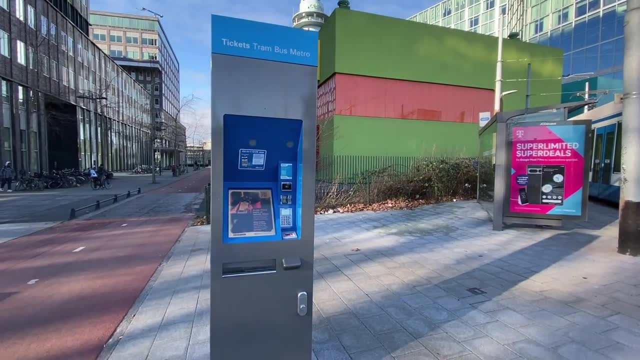 24-hour ticket. For the 24-hour ticket, you can buy this in a wide range of places, For example, from the driver on the bus or tram, from vending machines at metro stations, standalone vending machines at certain bus and tram stops, from a GVB kiosk, certain hotels. 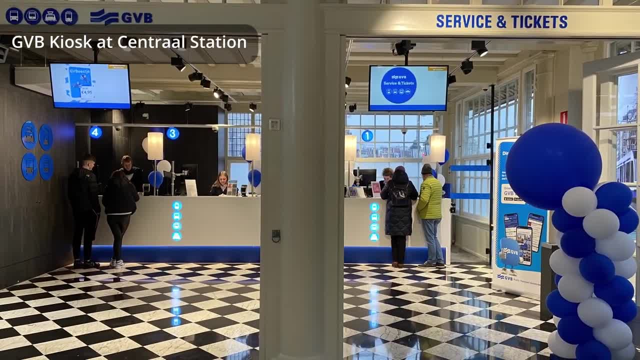 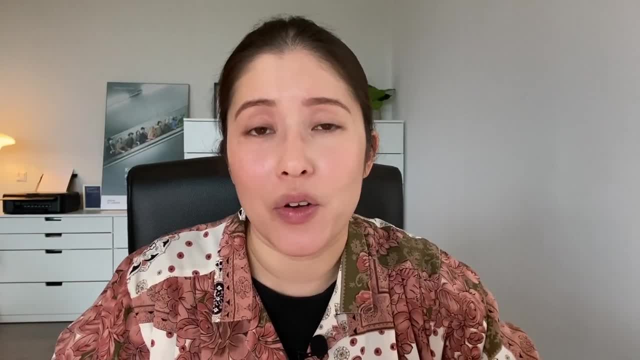 certain bookstores and online as well. Check out the GVB website for a full list of where you can buy this ticket. iAmsterdam City Card. Now, this card also varies in length of time, and you can get one that's 24 hours, 48 hours. 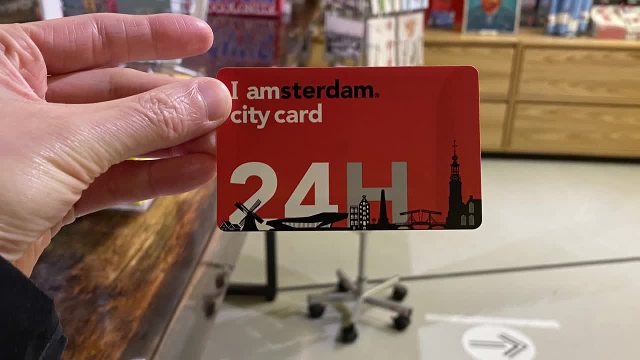 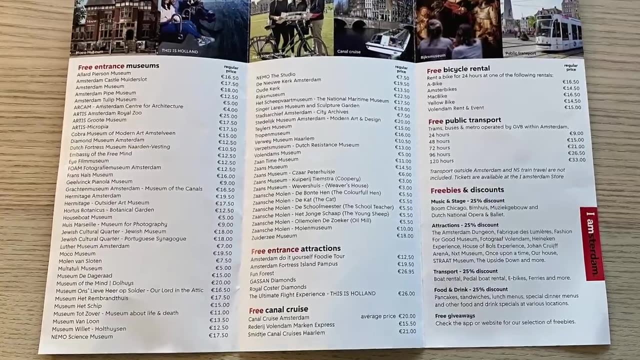 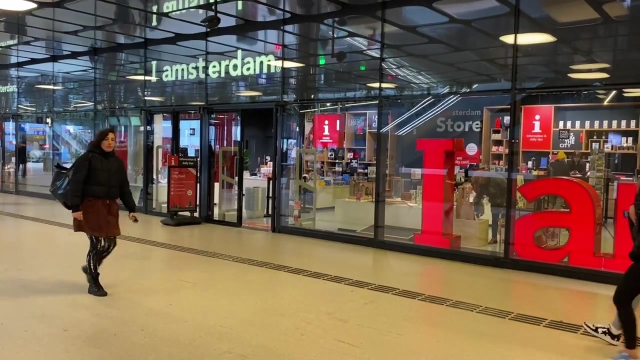 right up to 120 hours. The card will give you unlimited travel on the GVB network, free entrance to about 70 museums and attractions, as well as some additional freebies and discounts. You can buy this card online or at the iAmsterdam store, which is located at Central Station. 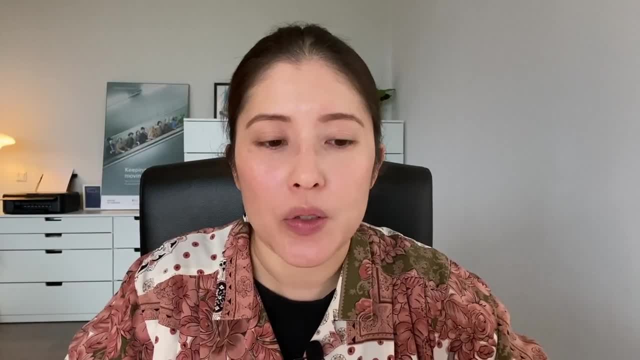 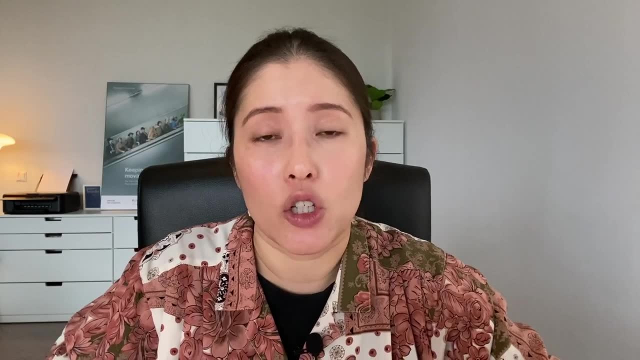 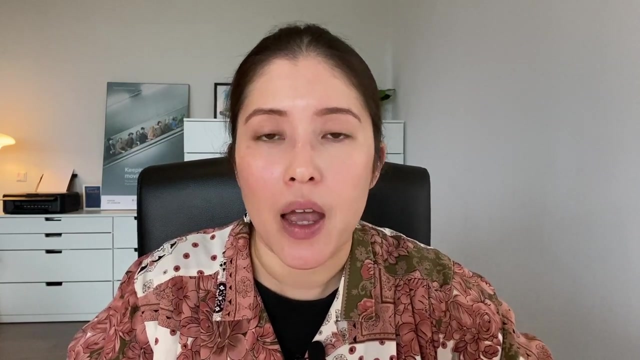 OV Chip Card. This is what you'll see most locals using. If you're visiting for a while or you live here, then it's definitely worth getting one. Basically, it's a smart card and you can put money onto it. The card costs €7.50 to purchase with a zero balance, and it will last. 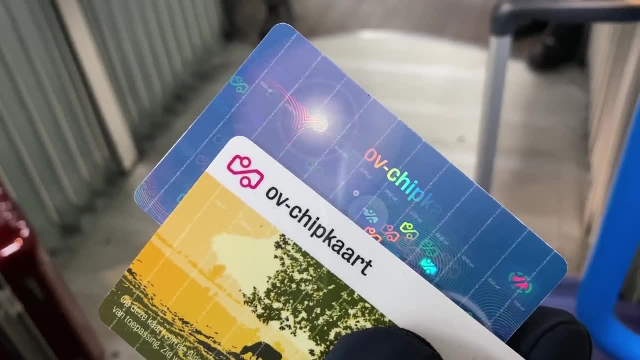 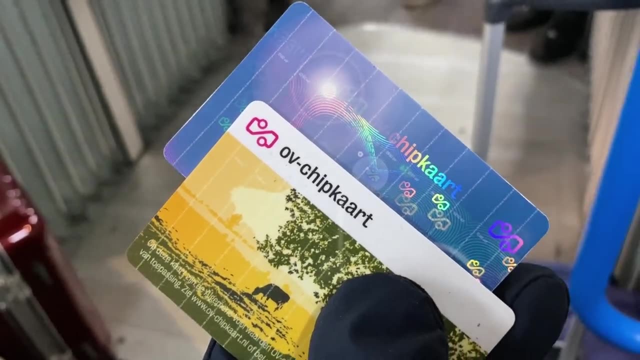 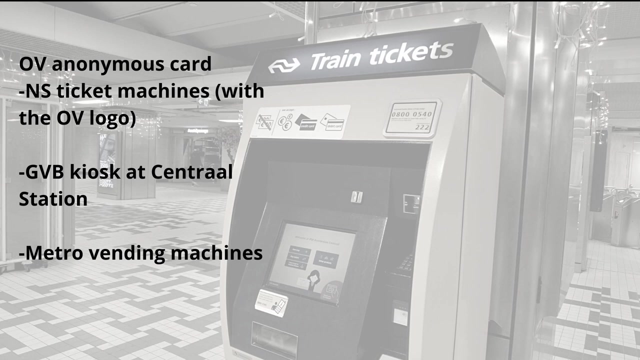 for five years. The blue one is an anonymous card so anybody can use this, whilst the yellow one is a personal card, so it will have, like, your name and your photo on it, And the anonymous card can be purchased from NS Ticket Machines, the GVB kiosk at Central Station and metro vending. 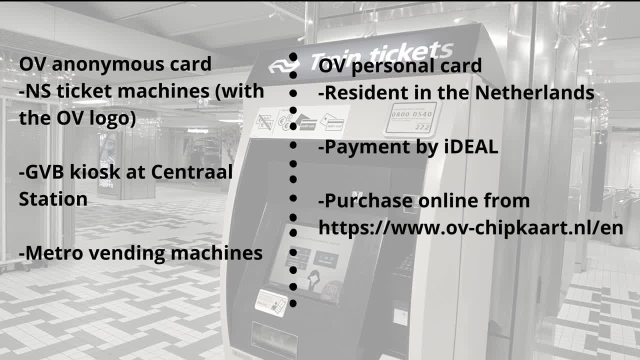 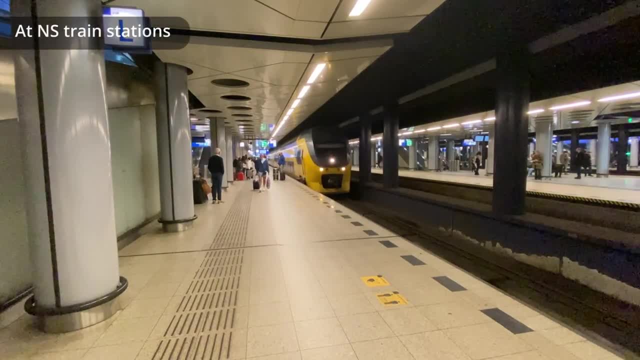 machines. Now, with the personal card, you need to be resident in the Netherlands and have a Dutch bank account, because payment can only be made with iDeal For train tickets. you can buy these at vending machines, service desks and also online. Now, another thing I wanted to mention. 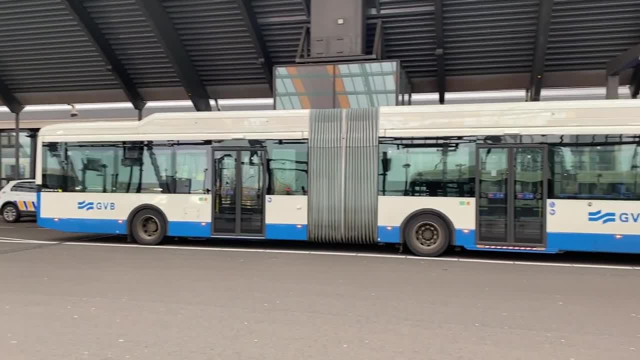 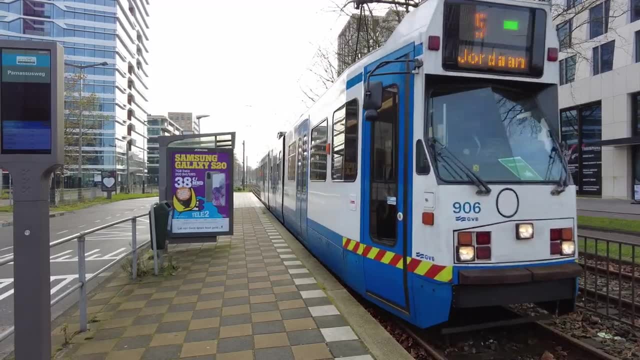 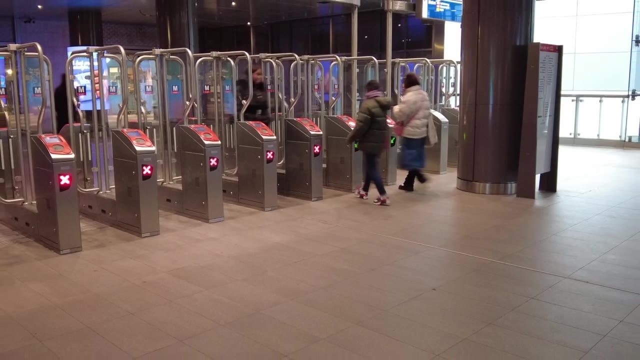 is something called OV Pay, and this is currently being rolled out on all forms of Dutch transportation and it's already available on the GVB network. What it means is that you can use your contactless debit card or credit card or mobile phone as a ticket and you literally just tap in and tap out and you're ready to go. So if you want to use this card online, you can use this card online and you can use this card online and you can use this card online and you can use. 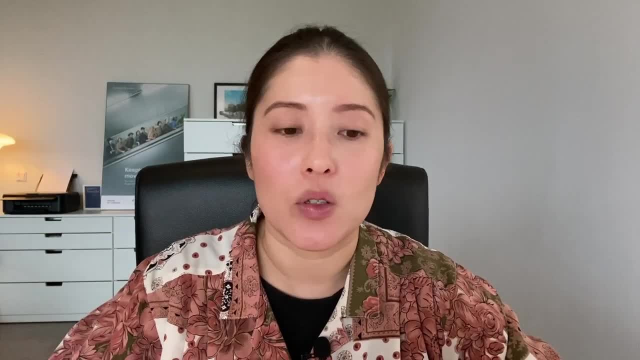 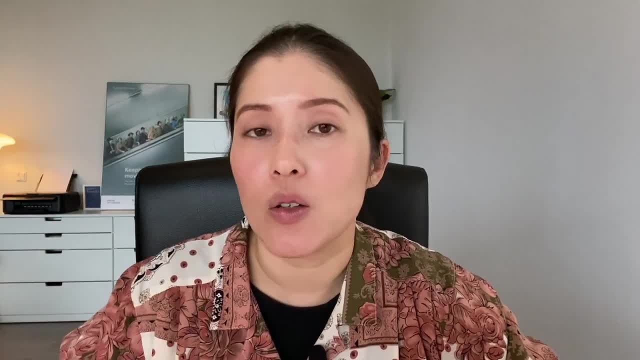 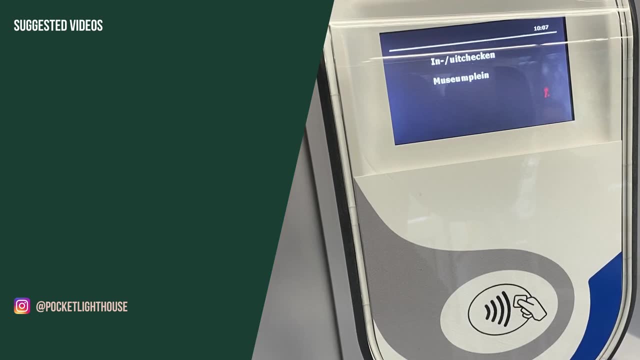 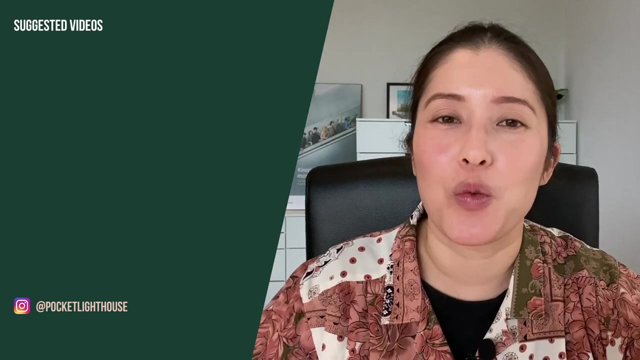 isn't working for some reason, then a quick way to find out where you are is to look at the ticket reader, because on the ticket reader it will say in or out, but it will also give you the name of the next stop so you can gauge where you are. I hope that's been useful. Thank you so much for watching. Until next time, goodbye.